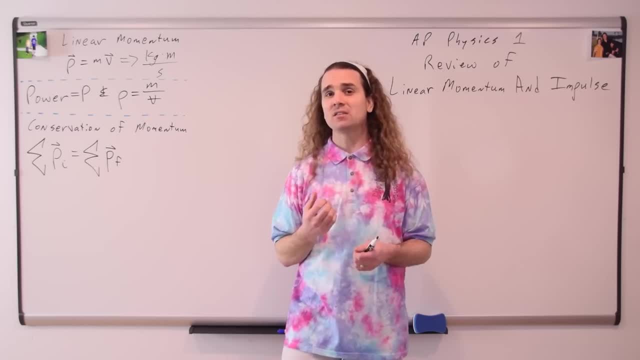 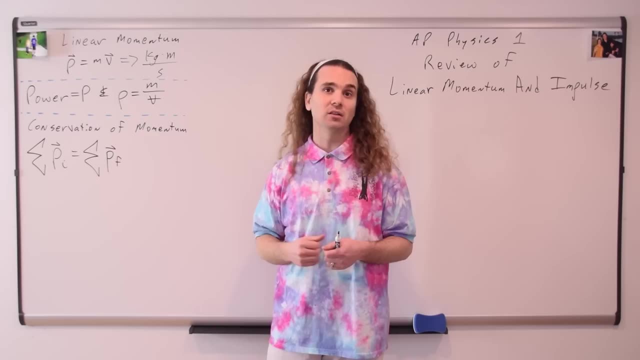 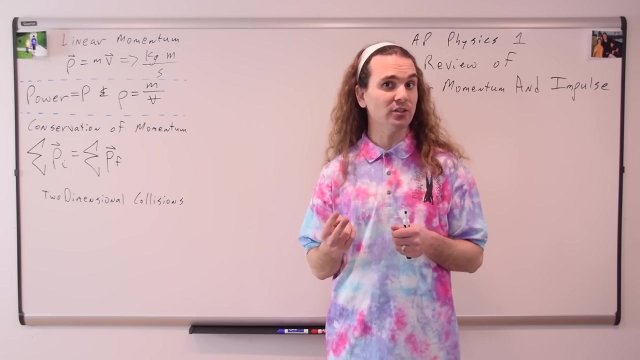 And, unlike conservation of energy, you do not need to identify the initial and final points, because the initial point is always right before and the final point is always right after the collision or explosion. Remember, momentum is a vector and if the objects are moving in two dimensions, 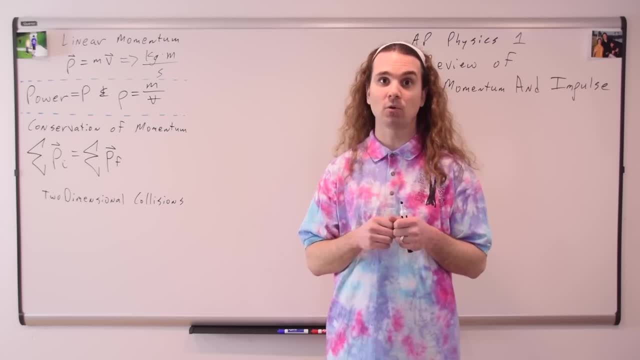 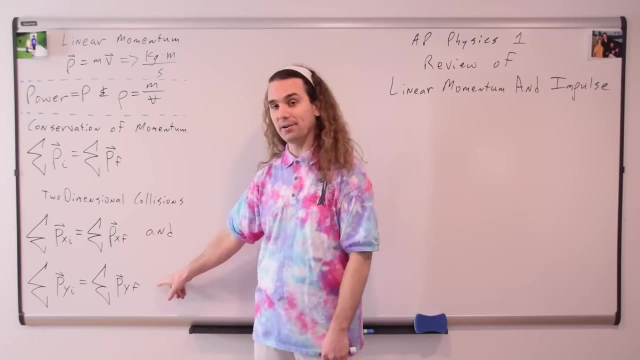 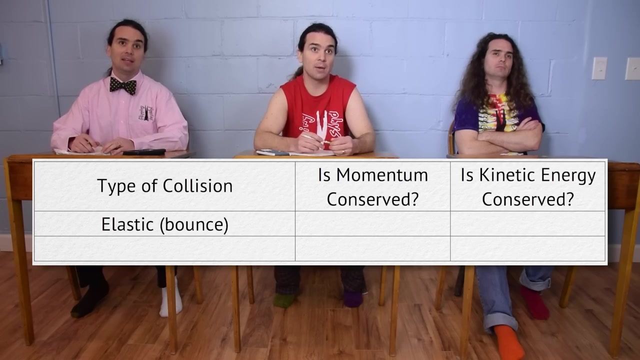 that means you need to have two different conservation of momentum equations, One for the x-direction and one for the y-direction. Bobby, what are the types of collisions? There is an elastic collision, where the objects bounce off of one another and both momentum and kinetic energy are conserved. 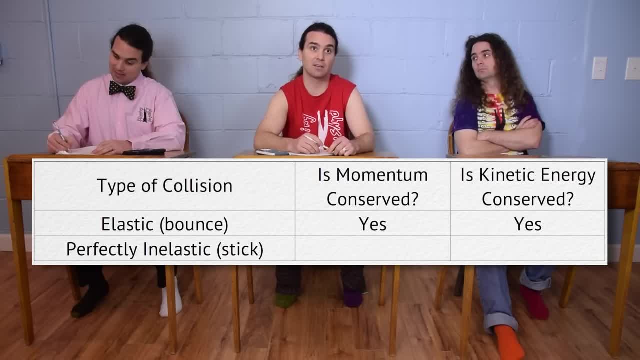 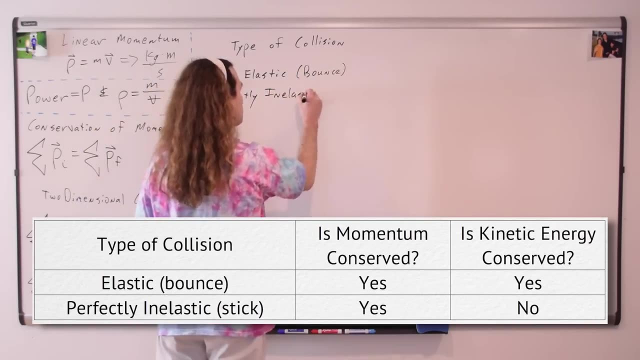 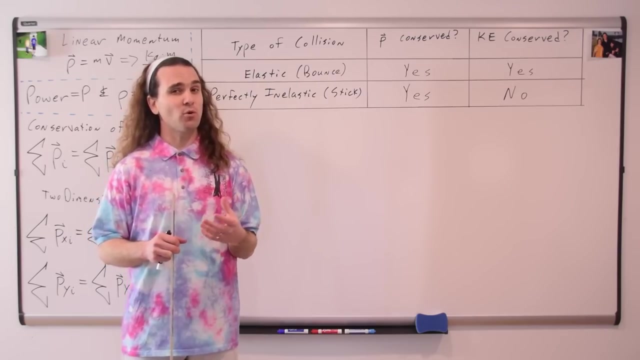 Then there is the perfectly inelastic collision, where the objects stick together and then move as one after the collision. In perfectly inelastic collisions, momentum is conserved and kinetic energy is not conserved. Many collisions are somewhere in between elastic collisions and perfectly inelastic collisions. 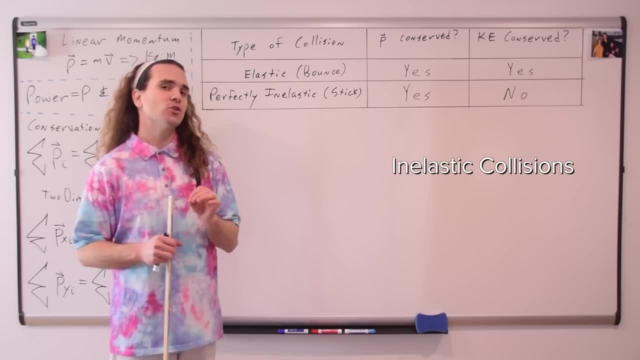 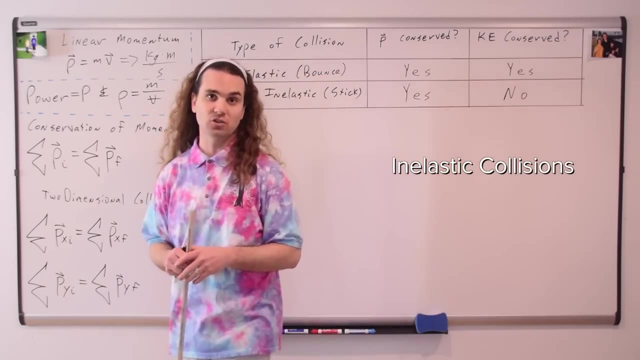 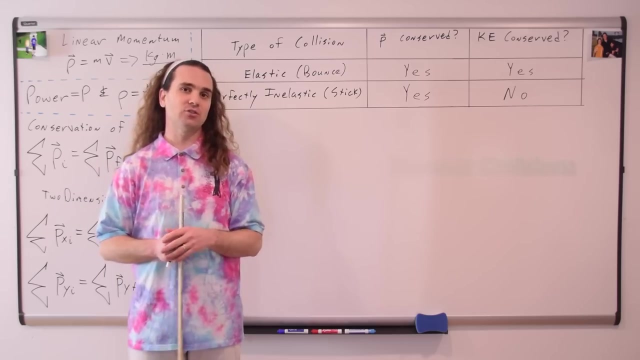 They are called inelastic collisions. During inelastic collisions, momentum is conserved. however, kinetic energy is not conserved. The elastic and perfectly inelastic collisions are basically the two ideal extremes. Okay, Let's go back to Newton's second law. 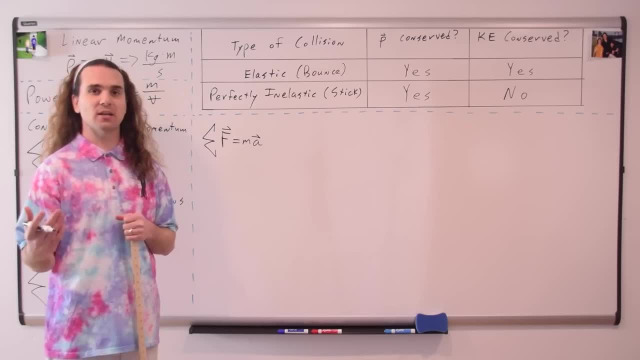 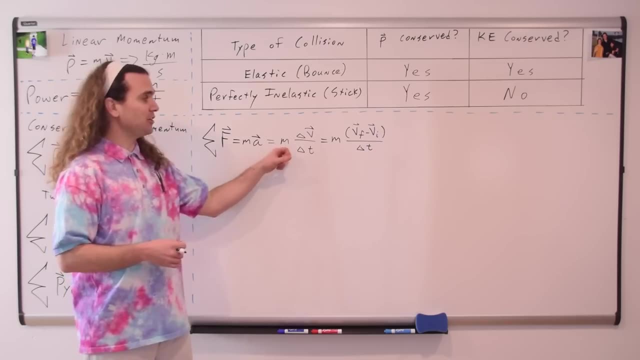 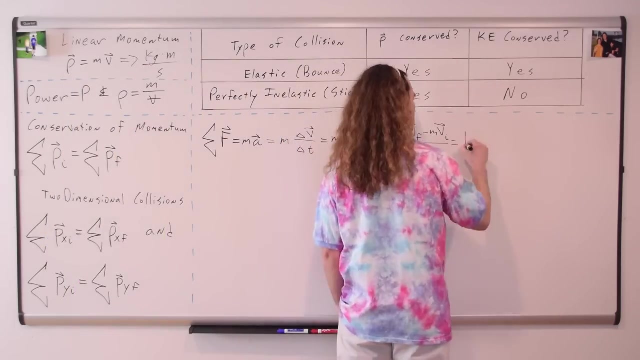 Net force equals mass times acceleration, where both force and acceleration are vectors. and now we can substitute in the equation for acceleration To get mass times change in velocity over change in time. and change in velocity is velocity final minus velocity initial. Multiply through by mass to get mass times. velocity final minus mass times, velocity initial. 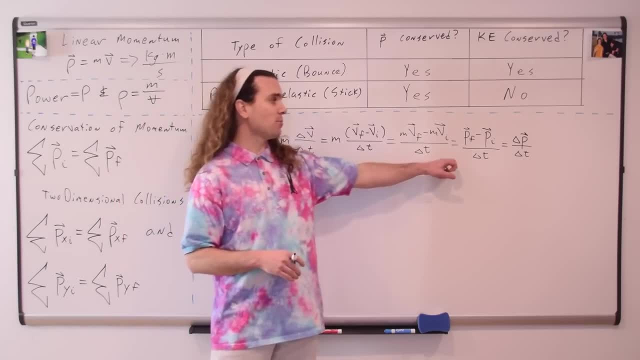 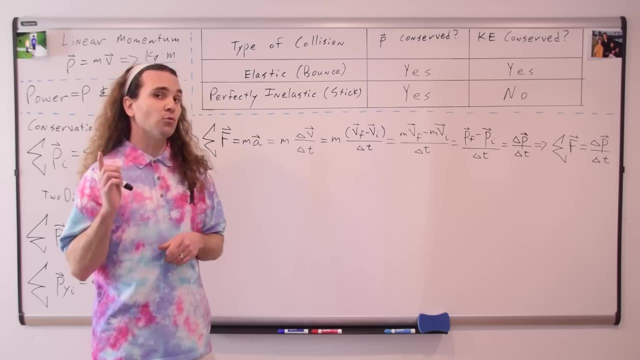 divided by the change in time, which is equal to the momentum final minus the momentum initial, divided by the change in time, which is the change in momentum over the change in time. In other words, a restatement of Newton's second law in terms of momentum. 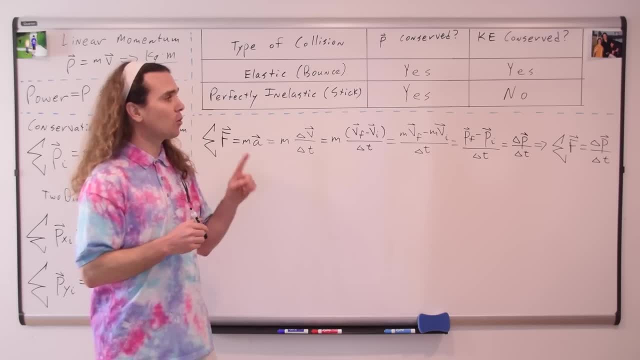 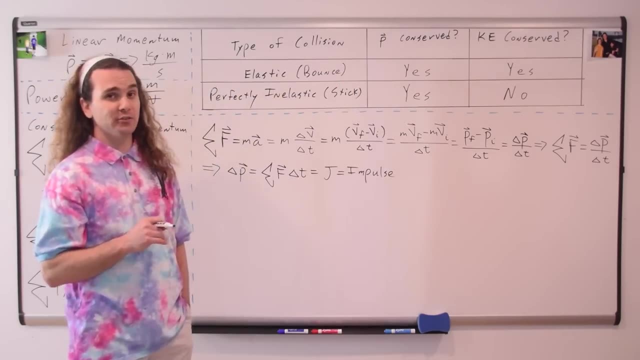 is that the sum of the forces equals the change in momentum over change in time, where both force and momentum are vectors. And if we rearrange the equation, we get the equation for impulse. Impulse equals the change in momentum, which equals the net force times the change in time. 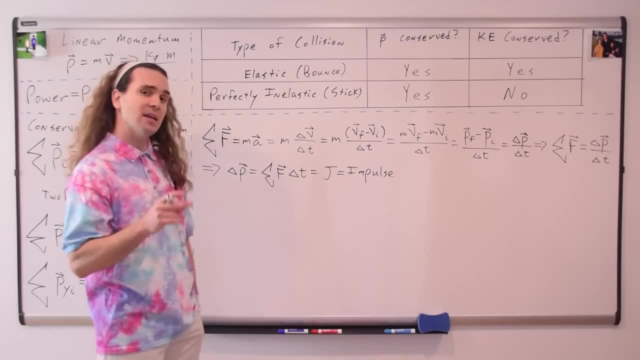 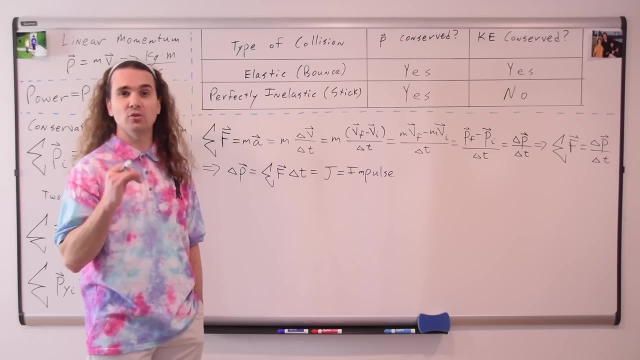 Typically the symbol for impulse is an uppercase J. Now this doesn't quite match the equation on your equation sheet for impulse. That's because generally during collisions we use something called the impulse approximation, which says that during the short time interval of the collision 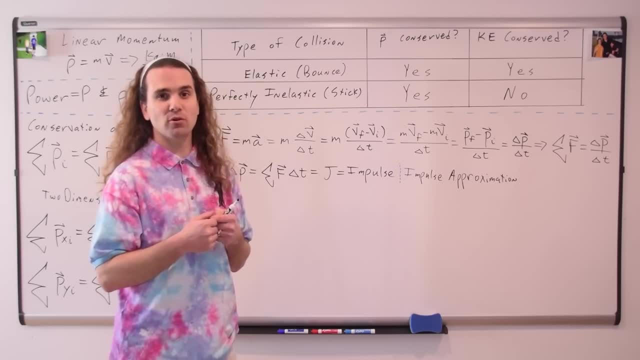 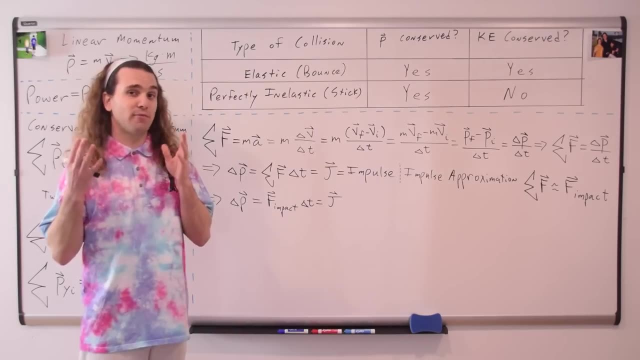 that force of impact is so much larger than the other forces that the net force can be approximated as the force of impact. Therefore, impulse is equal to the change in momentum, which is equal to the force of impact times, the change in time. 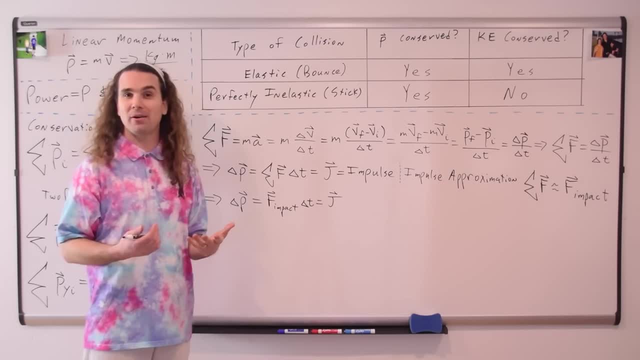 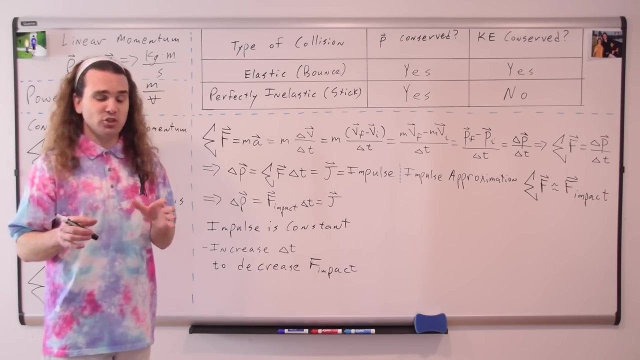 all during the collision. And the cool thing about impulse is this is how all of our safety equipment works: Safety belts, airbags, helmets, packaging foam- they're all based on the concept of impulse During a collision. an airbag doesn't change. 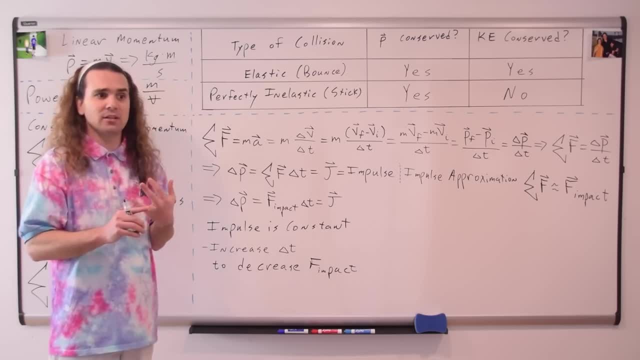 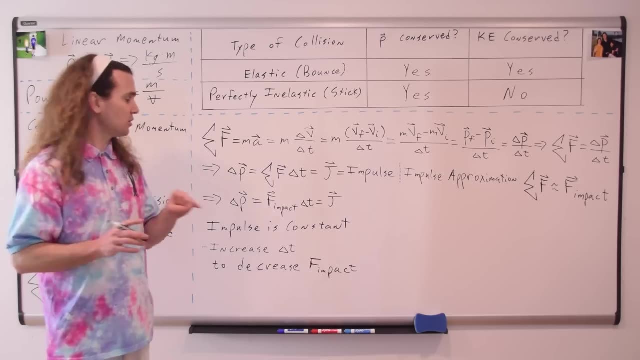 how fast your body was moving before the collision, how fast you're moving after the collision, or the mass of your body. So, regardless of whether you have an airbag or not, the impulse, the change in momentum of your body during that collision will be the same. 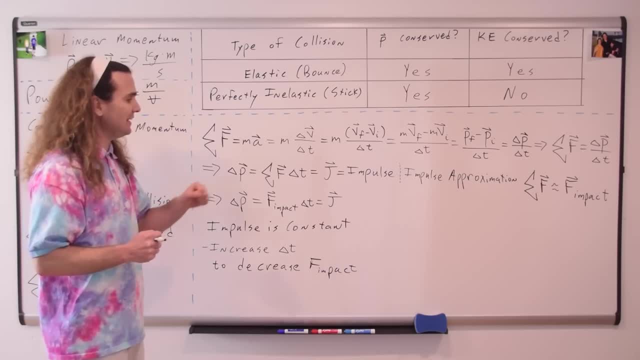 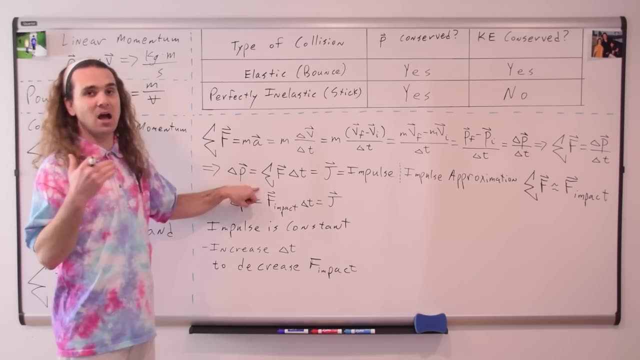 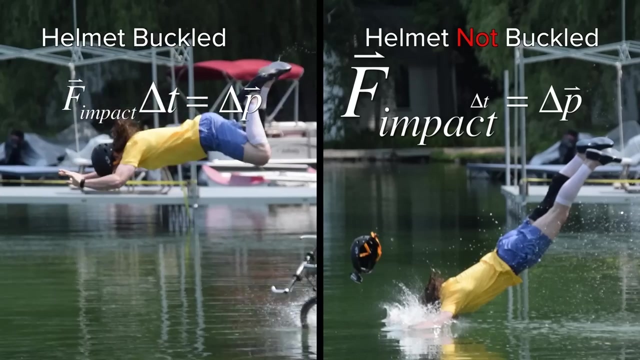 What an airbag does is: it increases the change in time of your body during that collision to then decrease the force of impact on your body during the collision. I actually rode my bike off of a dock into a lake several times to show this basic concept for a Flipping Physics video. 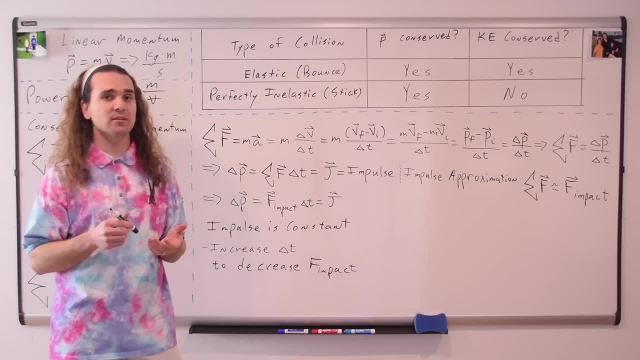 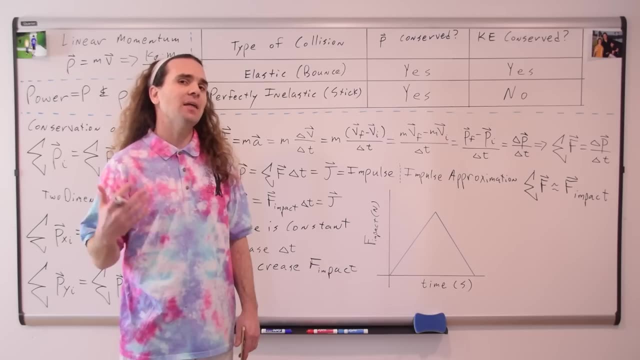 Now there will be times when the impact force is not constant. In that case, you can either use an airbag, use the average impact force, or you can use a graph, And the area between the curve and the time axis is the impulse. 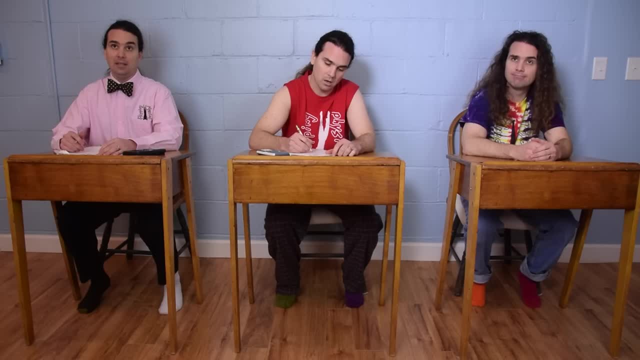 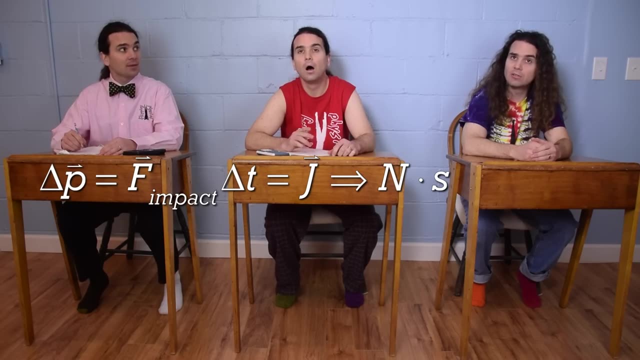 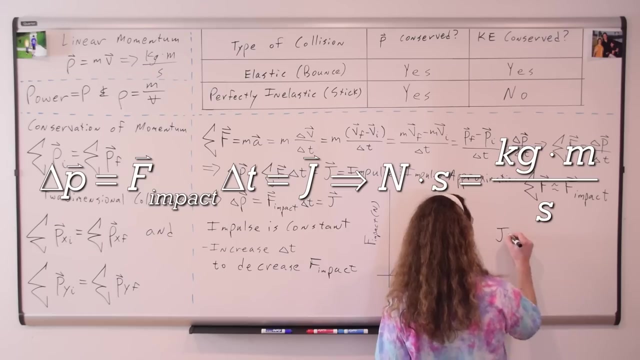 And Billy, what are the dimensions for impulse? Impulse is impact force. times change in time, so it is in newtons times seconds. Impulse is also equal to change in momentum, so impulse has the same dimensions as momentum, kilograms times meters per second.